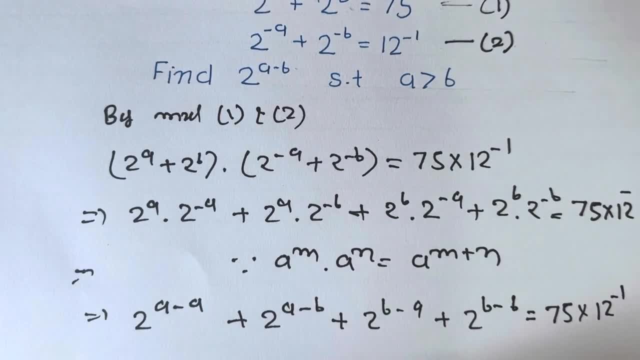 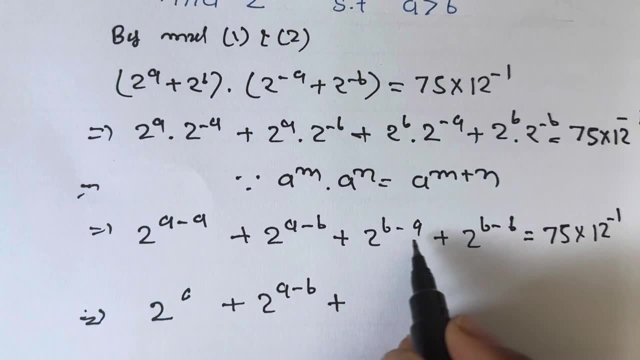 Which will be equal to to the power 0 plus to the power a minus b, and we can write to the power b minus a as 2, taking out minus 1 outside the bracket, and what is left, a minus b plus to the power b minus b, is equal to to the power 0 is equal to 75 into 12 to the power minus 1.. 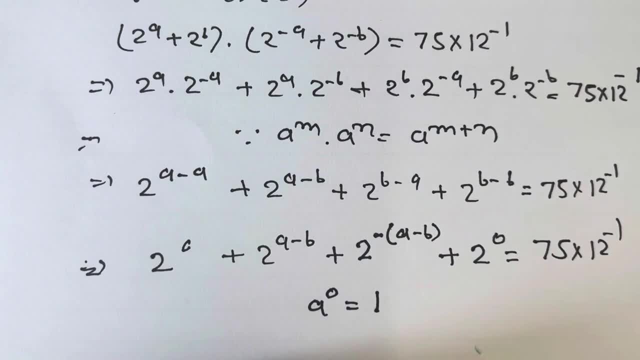 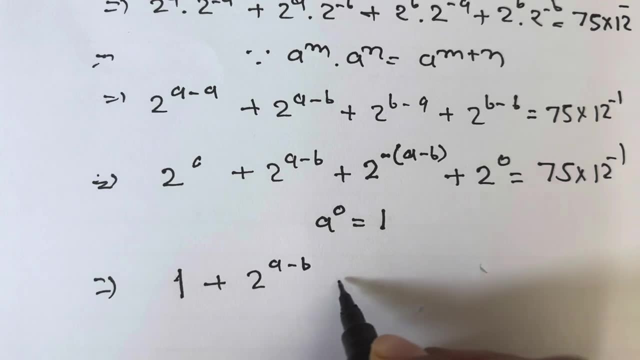 0th power of any number is equal to 1.. Hence this equation will become: 1 plus to the power a minus b plus to the power minus a minus b plus 1, equal to 75 into 12 to the power minus 1.. 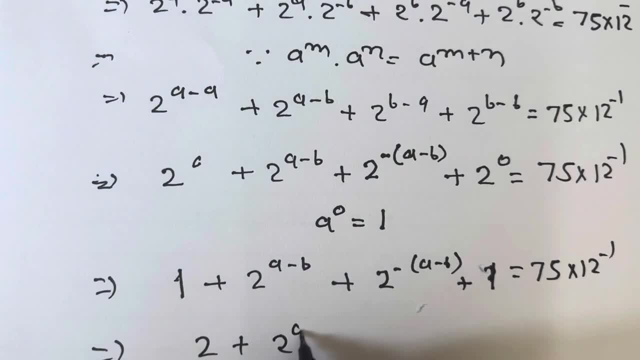 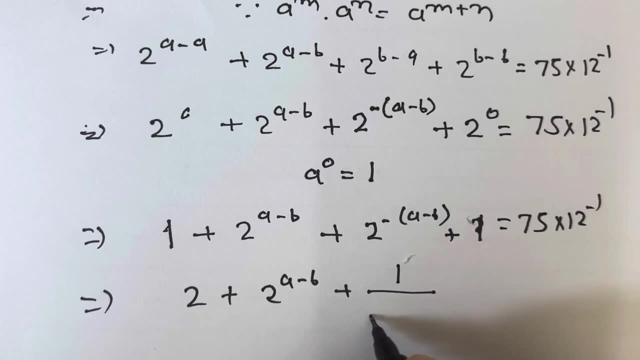 1 plus 1 is 2 plus to the power. a minus b. plus to the power minus a minus b can be written as 1 upon 2.. 1 plus 1 is 2 plus to the power a minus b. plus to the power a minus b is equal to 75, and 12 to the power minus 1 can be written as 1 by 12.. 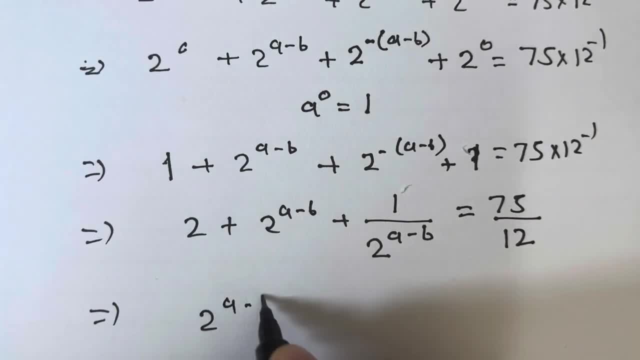 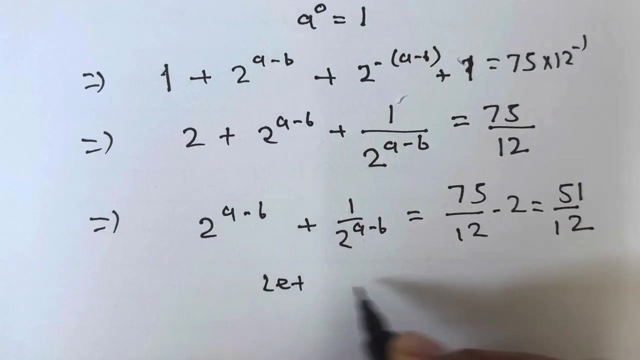 By simplifying this equation, we will get to the power a minus b. plus to the power a minus b is equal to 75 divided by 12 minus 2, which is equal to 51 by 12.. Now let us assume to the power a minus b is equal to x. 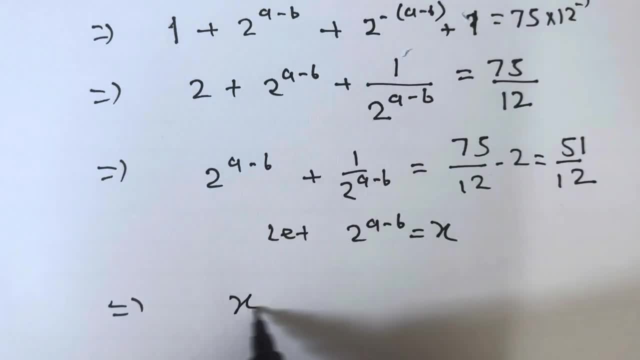 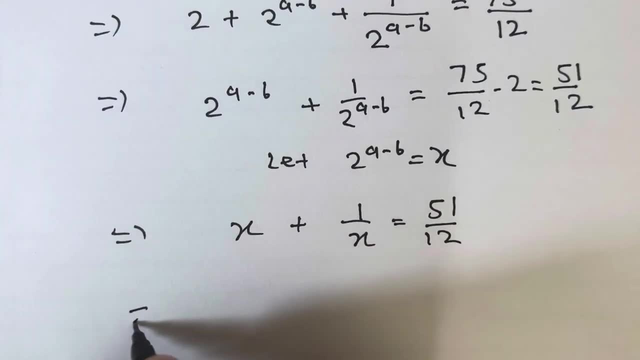 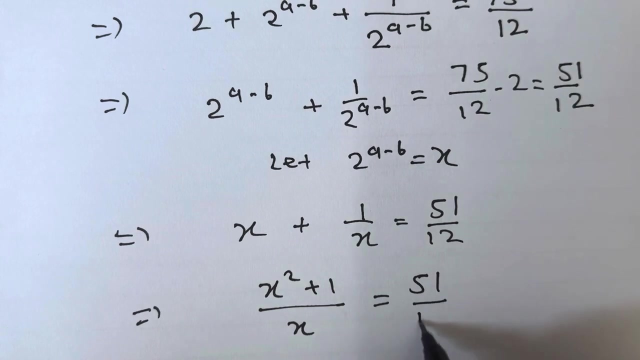 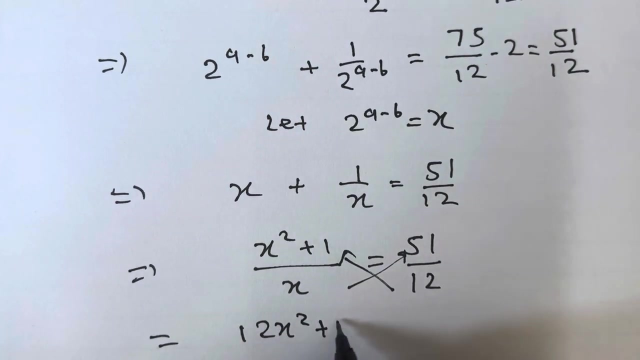 So the above equation will become: x plus 1 by x is equal to 51 by 12.. Now by simplifying further we will get x. x into x. x square plus 1 is equal to 51 by 12.. Now by cross multiplication we will get 12. x square plus 12 is equal to 51 x. 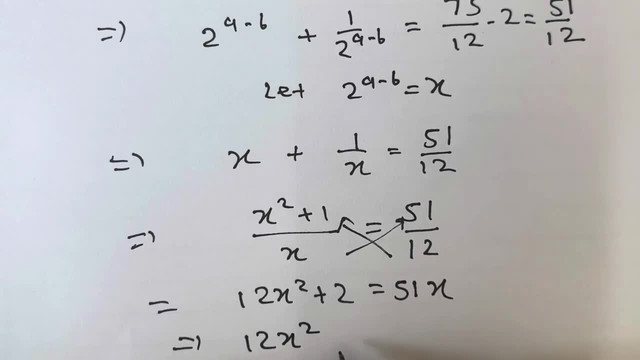 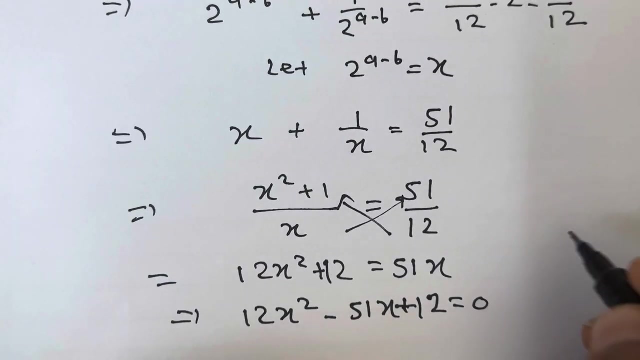 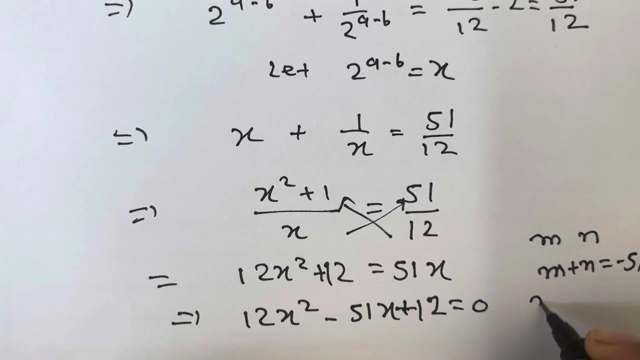 Can be written as 12 x square minus 51. x minus plus 12 is equal to 0.. Now to find the factors of this equation, we have to split minus 51 into two parts, m and n, such that the addition of that number should be equal to minus 51, and multiplication should be equal to 12 into 12, 144..